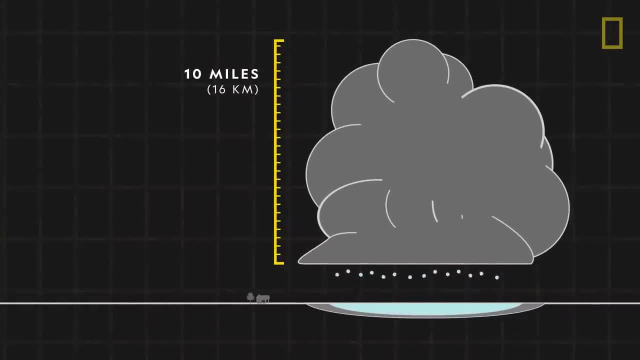 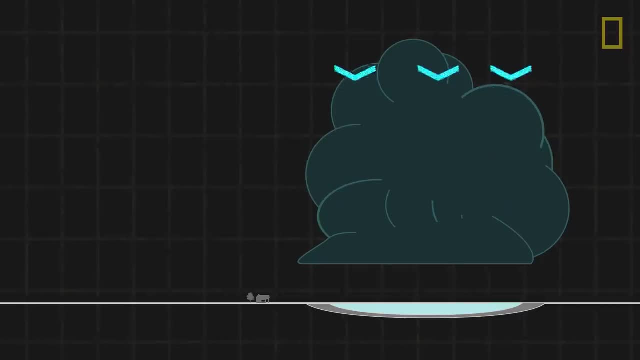 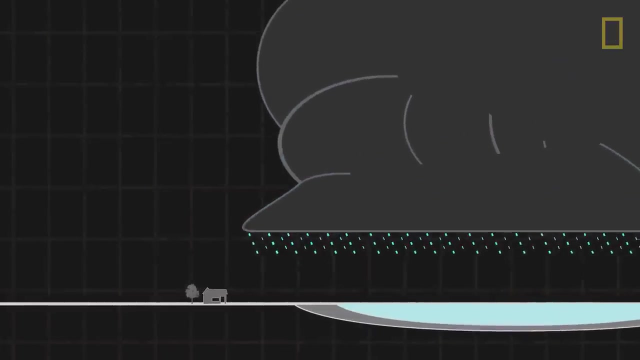 The clouds then build and grow, sometimes as tall as 10 miles high. The clouds darken as they fill and become heavy with water. Cool dry air from the upper layers of the atmosphere, known as a downdraft, then pull this moisture downward, causing it to fall as life-sustaining rain. In addition to helping sustain life, thunderstorms also help maintain the planet's balance of energy and electricity. When energy, specifically in the form of heat, causes water to evaporate, the heat is carried upward with a water vapor, As the vapor condenses and forms water droplets. 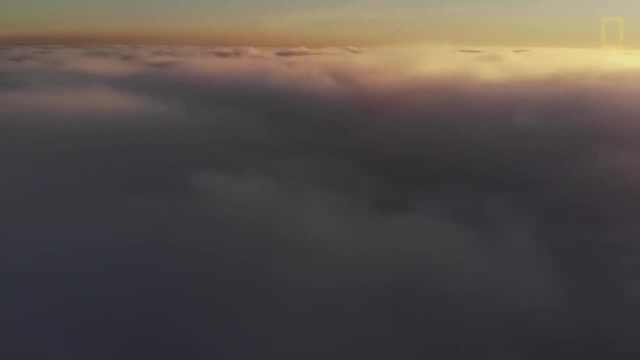 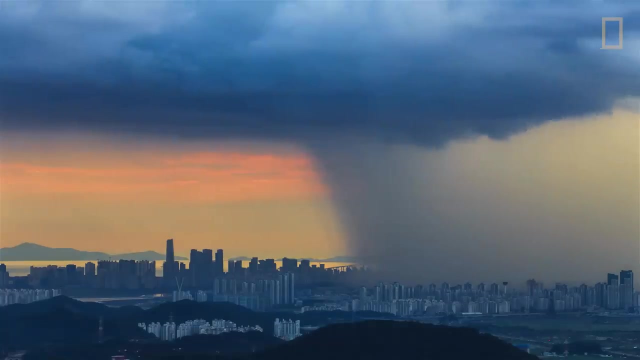 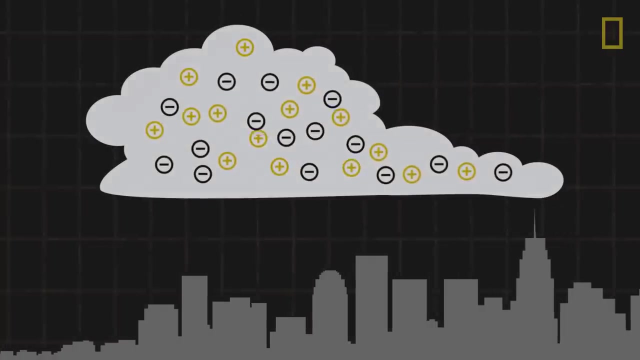 it releases the heat into the higher altitudes of the atmosphere and cools the Earth's surface. Thunderstorms also help regulate the electrical balance between the atmosphere and the planet. As clouds in a thunderstorm develop, excess positive and negative charges form within them. 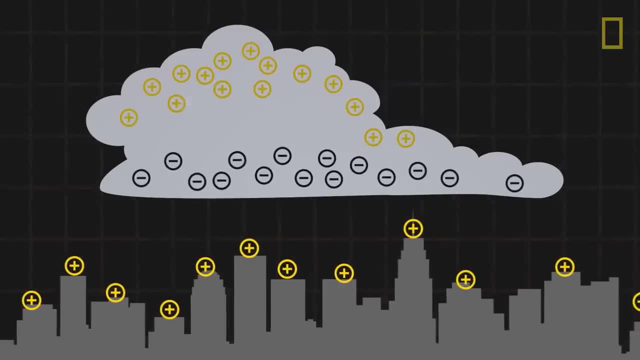 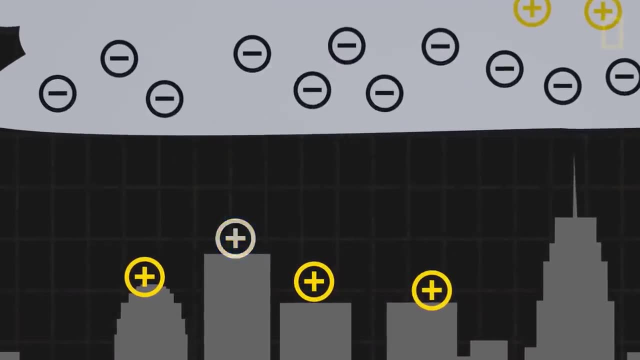 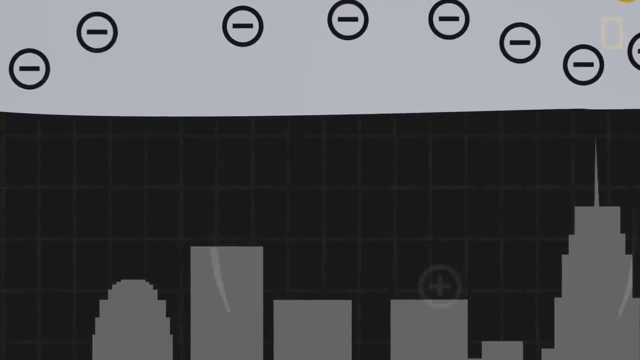 At a certain point, this buildup of opposite charges leads to the transfer of electrons in the form of lightning. This transference of electricity occurs so quickly that it breaks the sound barrier, a phenomenon that produces thunder, While thunderstorms are necessary for maintaining balance in the atmosphere. 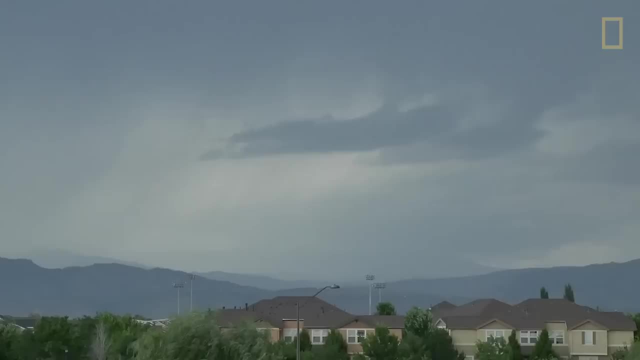 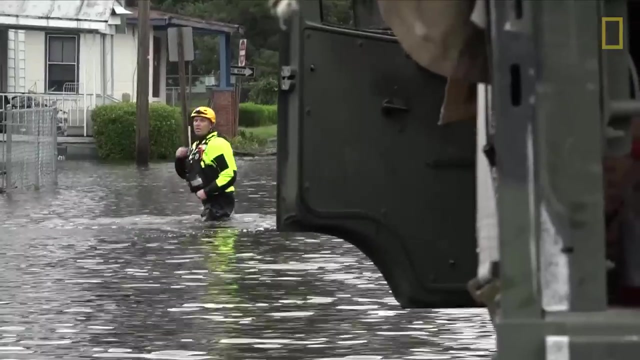 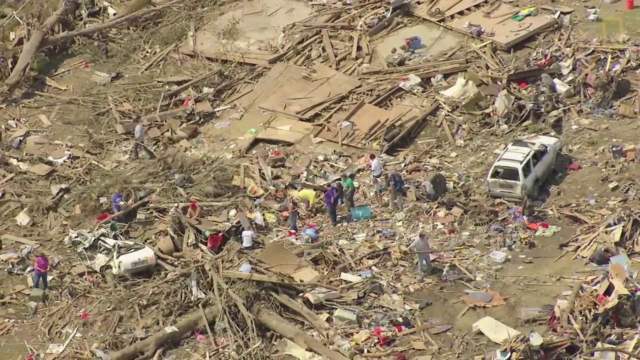 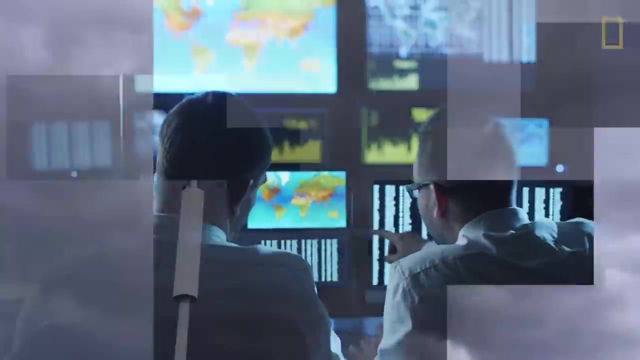 they can also be hazardous: Lightning strikes create fires, Excessive rainfall can cause flash flooding, and high-speed winds from tornadoes can destroy homes. Meteorologists study weather systems to try to predict the occurrence of thunderstorms and help ensure the safety of countless communities. 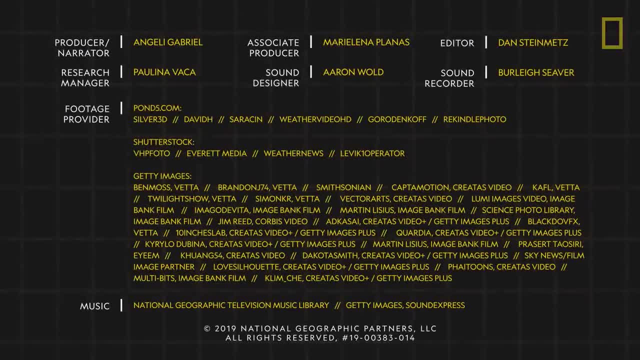 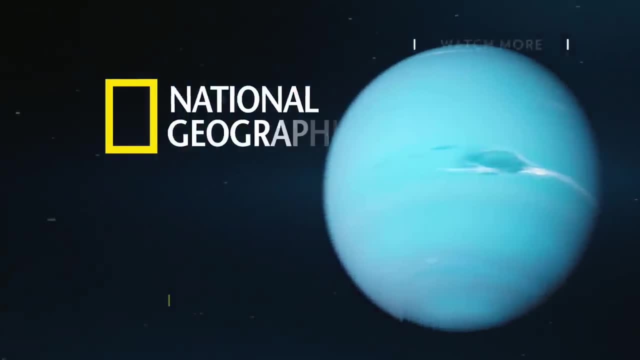 NASA Jet Propulsion Laboratory, California Institute of Technology. NASA Jet Propulsion Laboratory- California Institute of Technology. 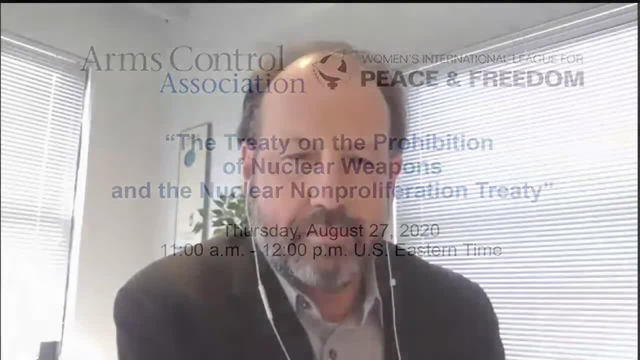 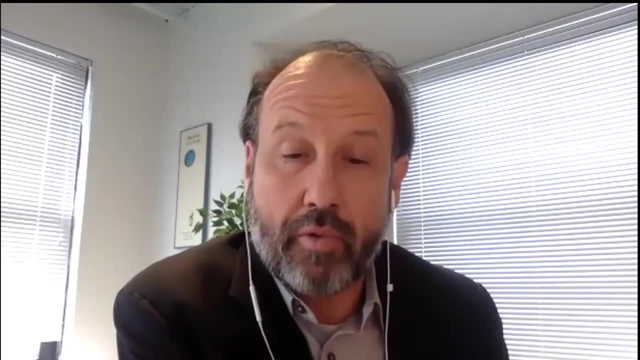 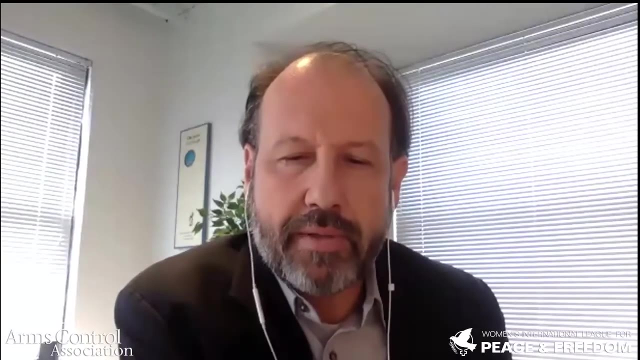 Good day everyone. My name is Darrell Kimball and I want to welcome everyone to the second of our Critical NPT Issues webinars, which are sponsored by the Arms Control Association and the Women's International League for Peace and Freedom. As I said, I'm Darrell Kimball. 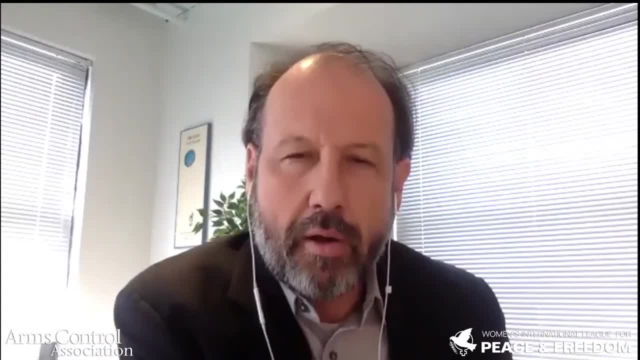 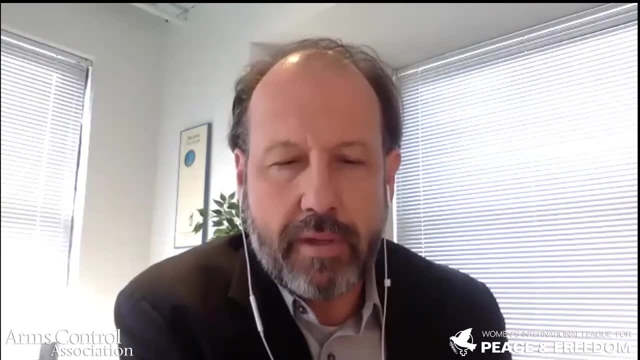 with the Arms Control Association. I'll be the moderator today for our discussion on the Treaty on the Prohibition of Nuclear Weapons and the Nuclear Nonproliferation Treaty. As many of you know, the pivotal 10th review conference of the NPT has been rescheduled and will most likely be.